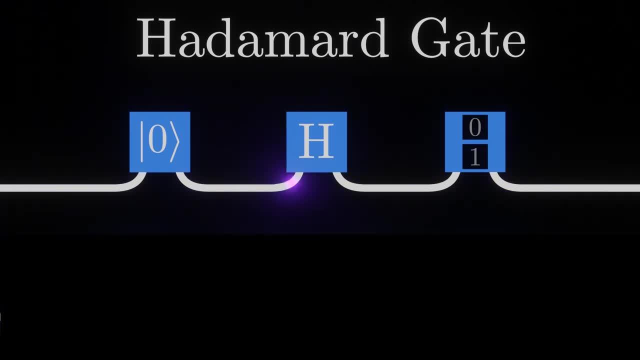 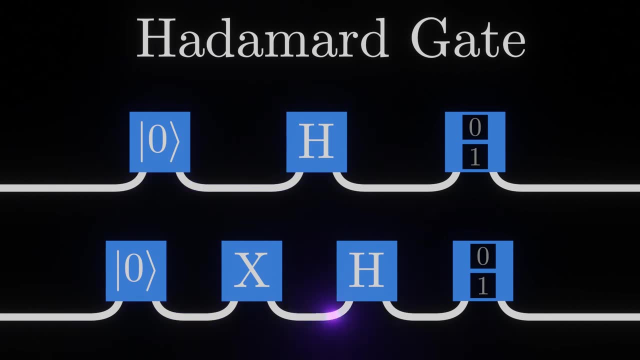 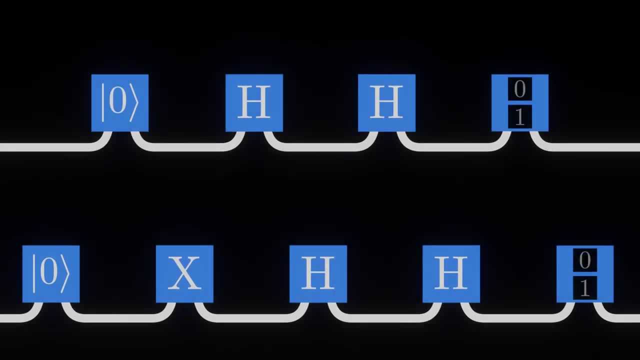 and half the time we measure it as 1.. The same thing happens if we use a qubit starting in the 1 state. From this, it might seem like the H gate is just randomizing the qubit. If this was the case, we'd expect that two H gates in a row would have the same effect. 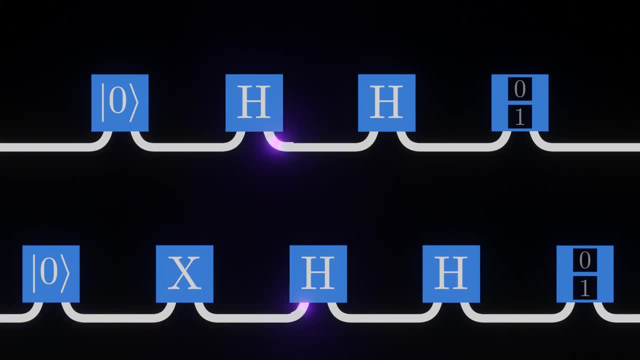 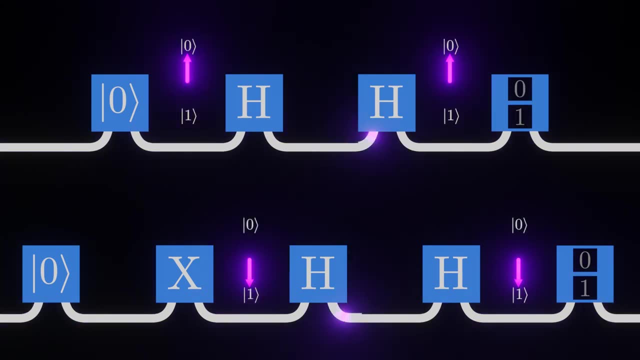 the second gate, just randomizing the qubit a second time. But when we perform this experiment, we find that the qubit is always measured as whatever it started, as What this tells us is that the qubit carries more information than just whether it's 0 or 1.. 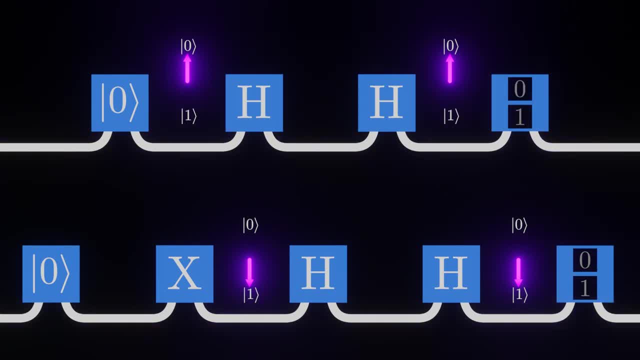 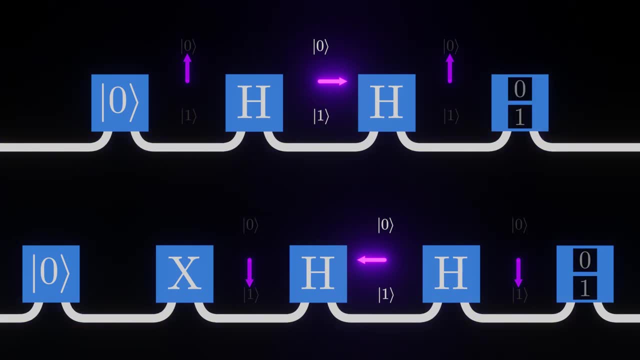 More specifically, it's useful to say that in between the two H gates, the qubit remembers that it's in between the 0 and 1 states. A qubit with some kind of in-between state like this is said to be in a superposition. 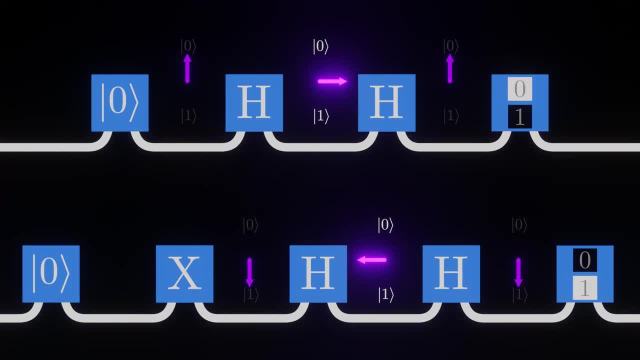 You can think of this notation as saying that this qubit is equally likely to be measured as 0 or 1, instead of just being 100% likely to be measured as 0, or 100% likely to be measured as 1.. 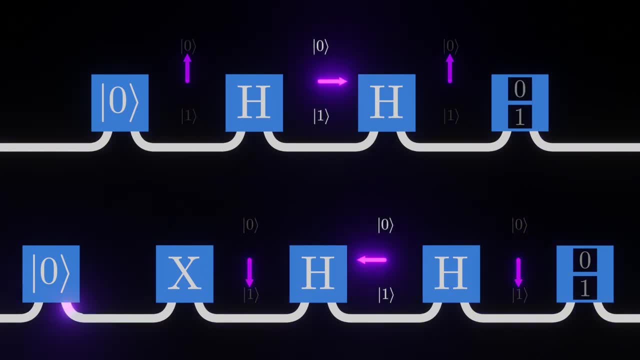 The H gate turns 0 and 1 qubits into two different kinds of superpositions, allowing the second H gate to correctly undo the effect of the first. Notice, though, that each of these superpositions have the same chances of being 0 and 1,. 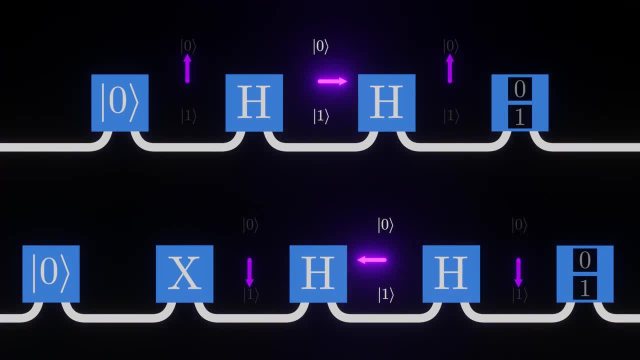 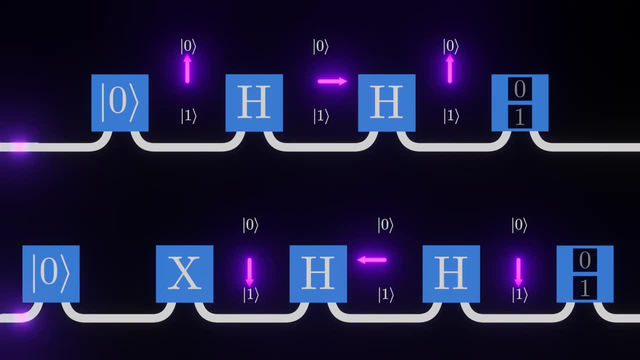 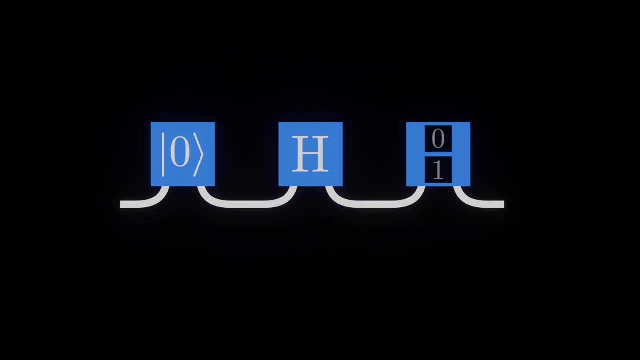 explaining why we didn't notice this effect when we measured after the first H gate. Let's now use this effect to get a better understanding of the measurement. Like we saw before, placing a measurement after an H gate produces random results. This makes some amount of sense. 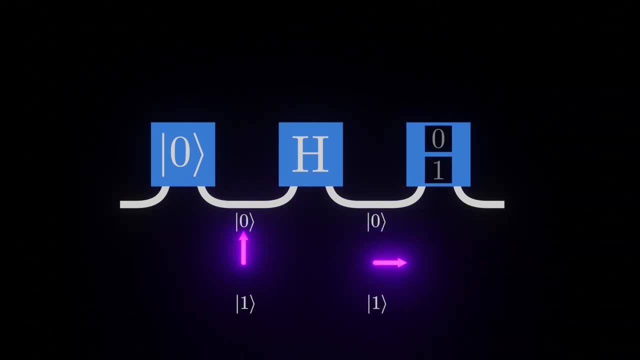 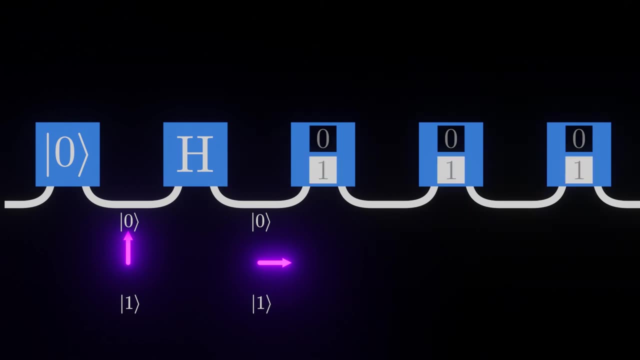 because it's the most accurate picture we can get of the superposition with such a blunt measurement. Let's now try placing a few measurements in a row. Surprisingly, they always agree with each other. This tells us that the measurement isn't just. 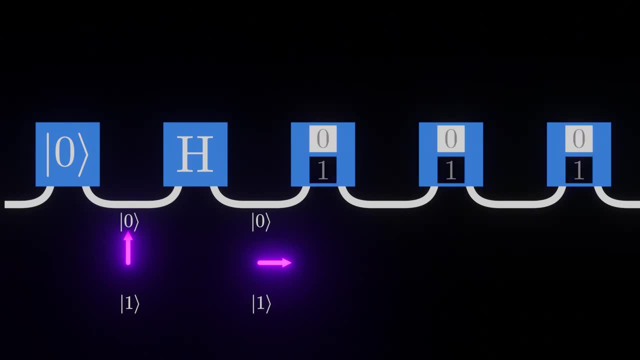 randomly reporting some possible state each time. If it were, we'd expect the results of each gate to be uncorrelated. We'd expect each measurement to act like an independent coin flip, paying no attention to the other's results. This tells us that the measurement isn't just passively noting things down. 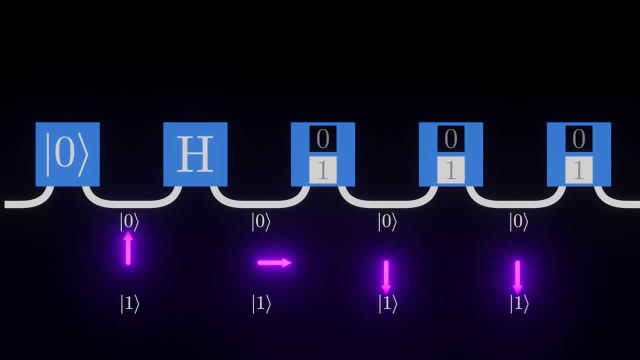 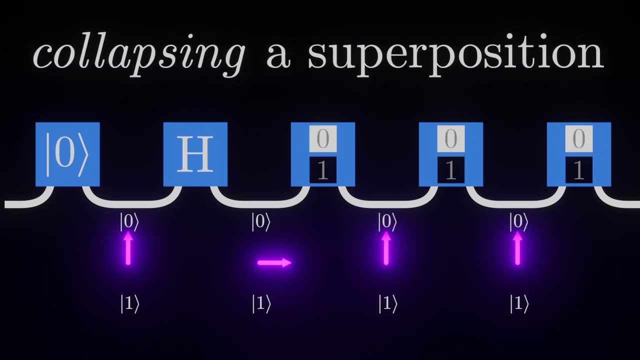 but is actively changing the state of any qubit it touches, such that later measurements produce the same result. Specifically, the measurement gate works by randomly selecting one of the possible states, then making that the only possible state. This effect is called collapsing a superposition. 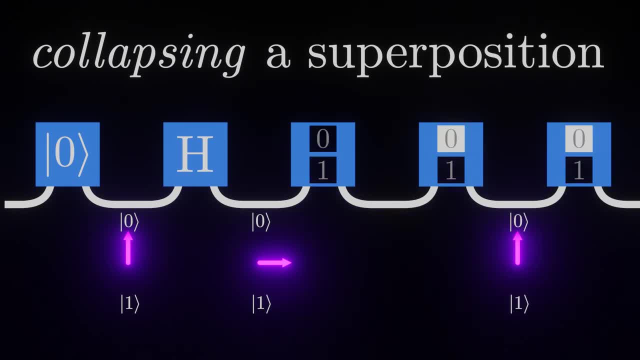 The reason we still call this the measurement gate and not the collapsing gate is because there's no known way to directly measure the properties of a superposition without collapsing it. By doing this with a measurement gate, we learn what specific state the superposition collapsed to. 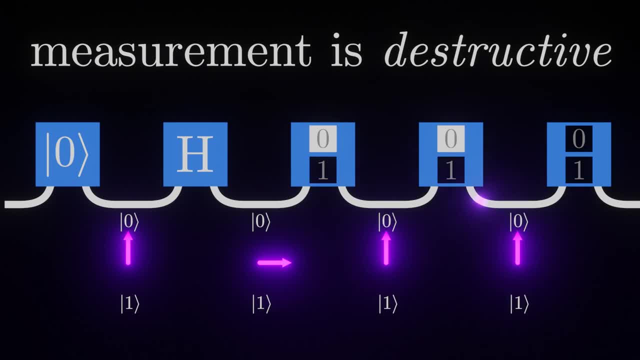 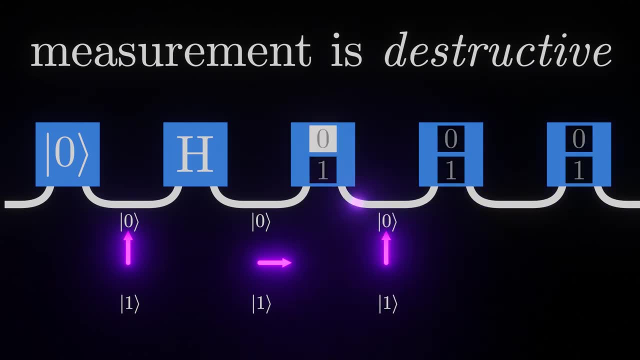 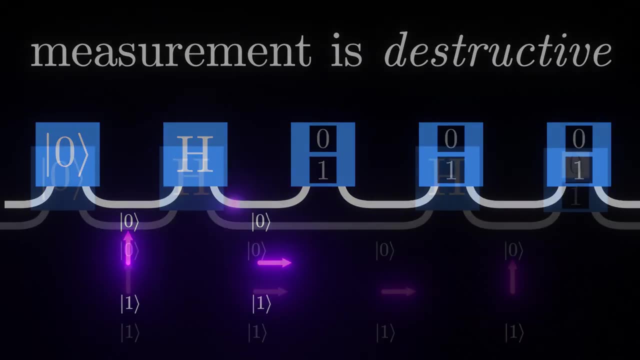 This is also why we say that measurement is destructive. The process of measuring a qubit destroys some of the information it carries. This explanation suggests an interesting experiment to prove the properties we found Before we saw that: passing a qubit through two atomar gates. 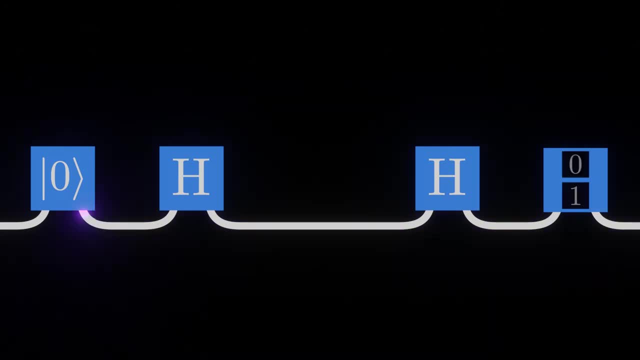 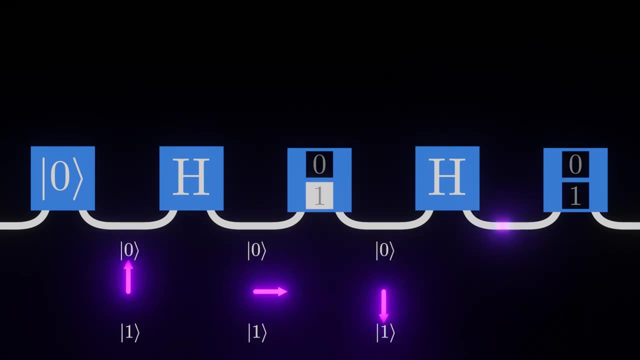 causes it to remain unchanged. Let's see what happens when we put a measurement gate between the two H-gates. Since the measurement collapses the qubit, we see that the second H-gate now appears to randomize the qubit just like the first. 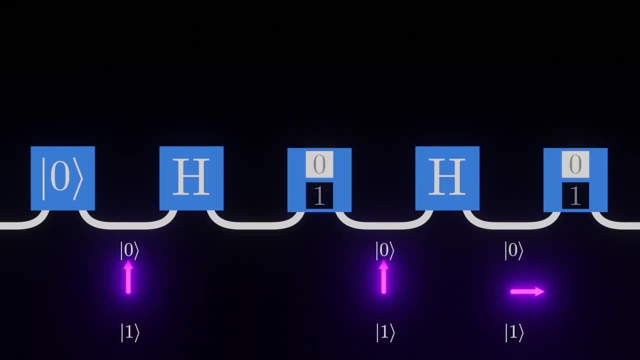 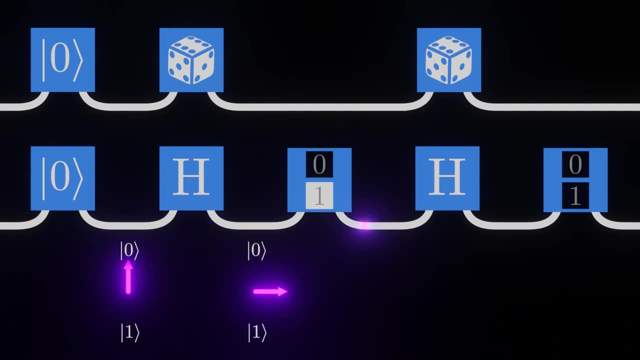 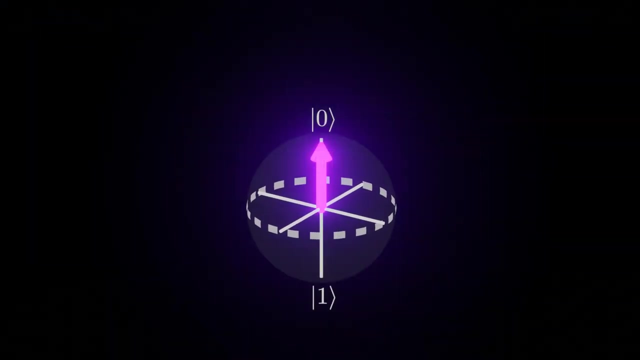 Recall that this mirrors the behavior we would expect if the H-gate by itself acted like a randomizer. This tells us that the randomness we see is not a property of the H-gate itself, but a property of measurement. Let's take a step back to formalize some of our definitions. 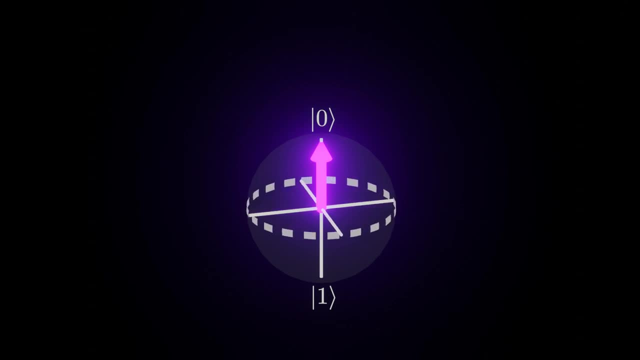 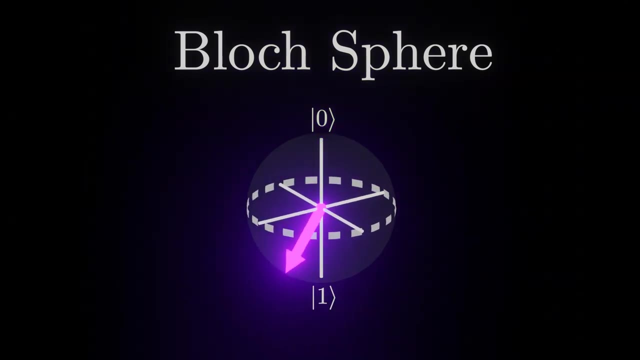 The notation we've been using so far to represent the state of a qubit is called a Bloch sphere, although we've been using it as more of a Bloch square so far. This handy diagram represents all possible states a qubit can be in as points on a sphere. 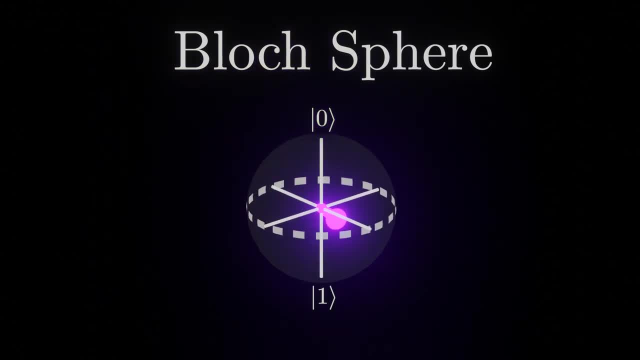 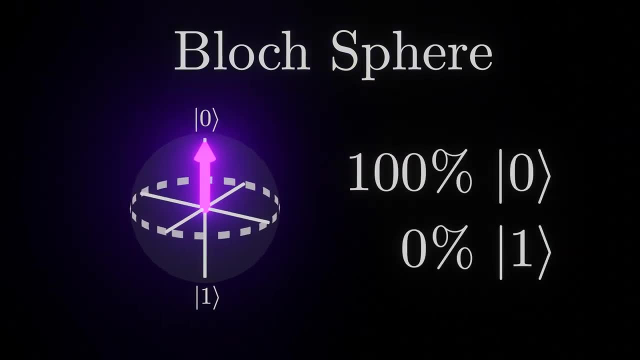 We usually draw an arrow from the center of the sphere to make the diagram easier to read. An arrow pointing up represents a qubit that will always be measured as 0, and an arrow pointing down represents a qubit always measured as 1.. 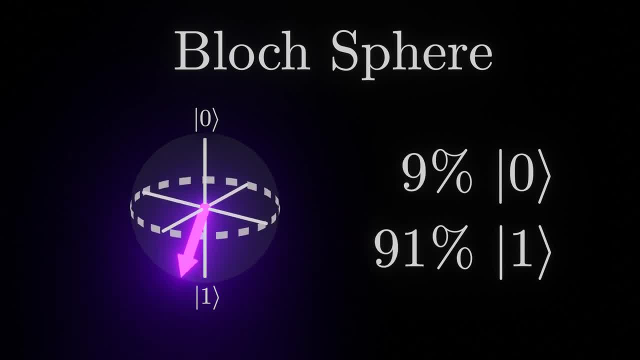 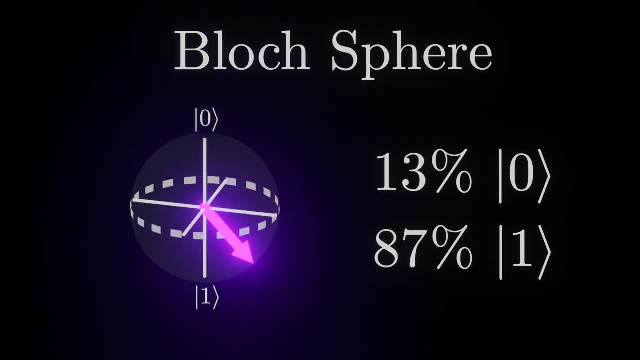 In general, the likelihood of a qubit to be measured as 0 or 1 is represented by how much its analogous Bloch sphere is pointing in that particular direction. All the logic gates we've looked at and the ones we have yet to cover. 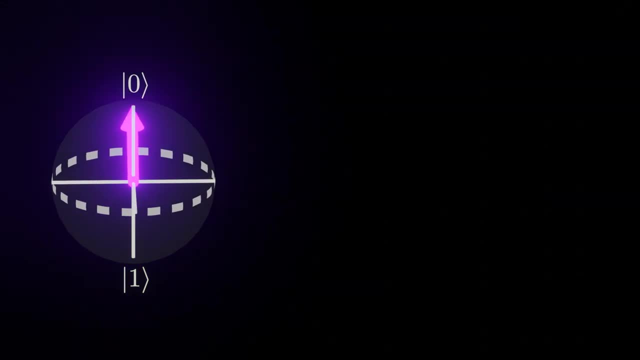 act analogously to some rotation on the Bloch sphere. Because of this, it's helpful to label a few axes as points of reference. From this labeling we can see where the x-gate gets its name. Specifically, its function can be described. 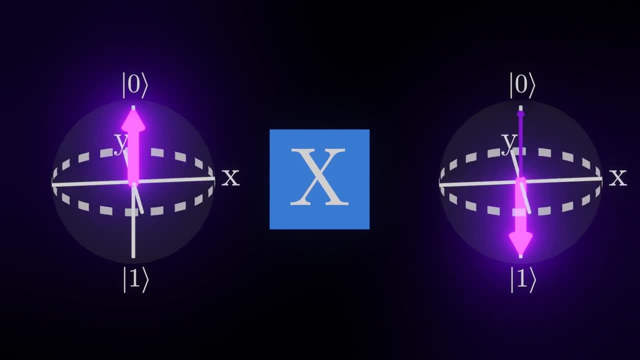 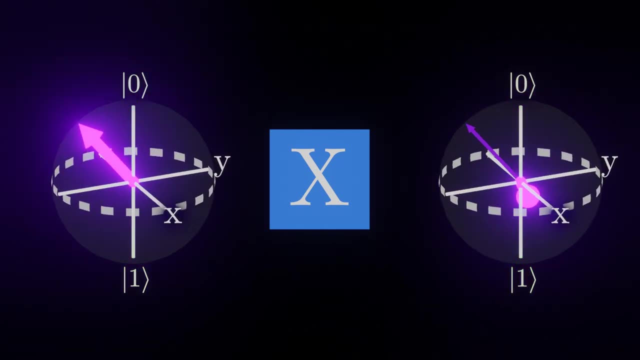 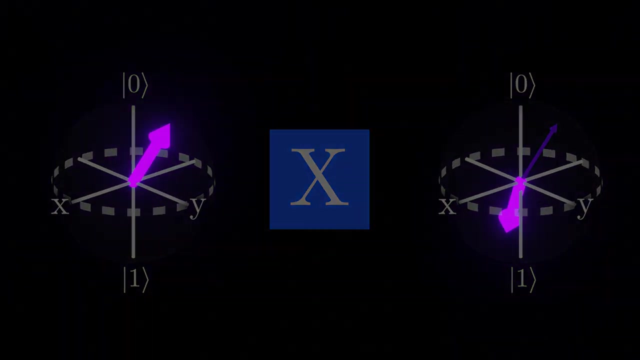 as a half rotation around the x-axis. Notice how this flips a 0 qubit to 1, and vice versa. This also tells us what happens in cases where the qubit is not exactly 0 or 1.. The predictably named y- and z-gates. 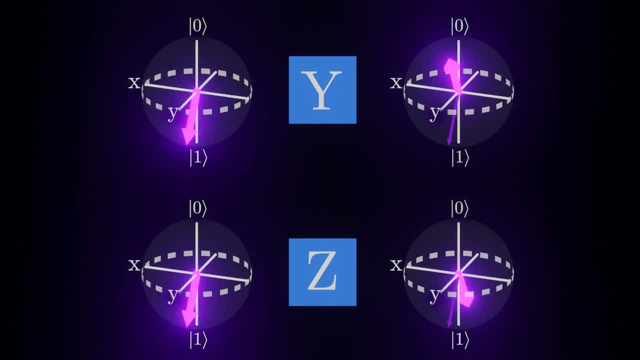 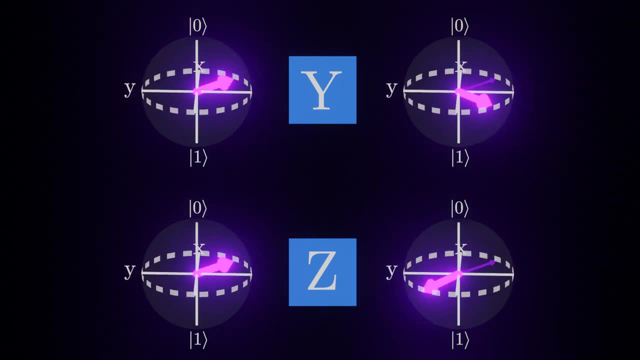 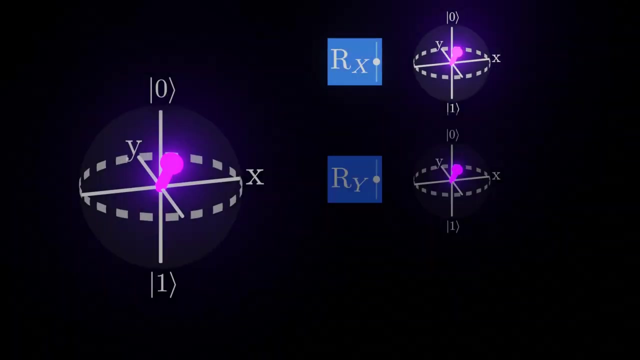 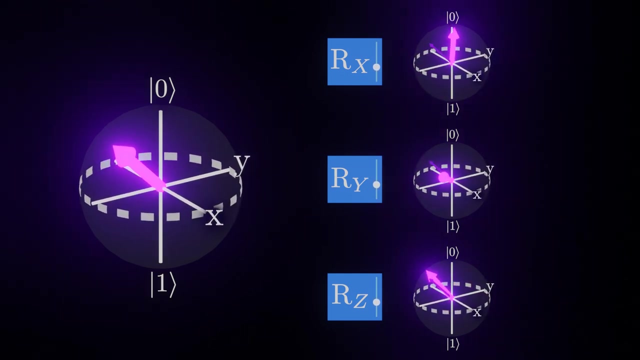 perform the same function around their respective axes. More generally, we can talk about our x, our y and our z-gates that rotate along these axes by some specific amount that we get to pick. For example, we could describe an ry-gate. 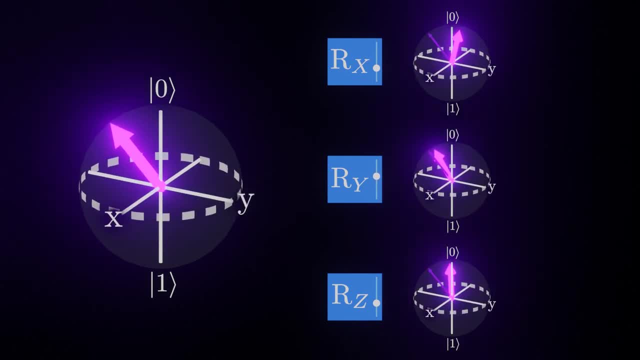 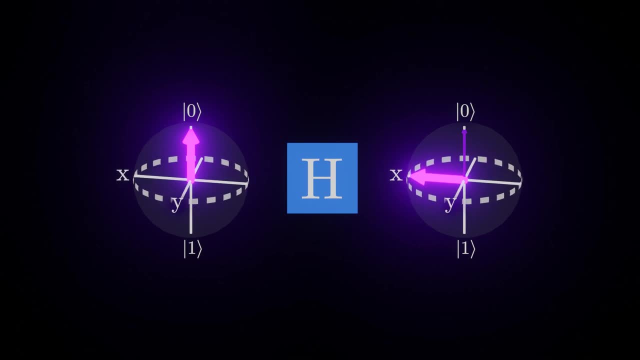 that rotates by half a radian, or maybe an rx-gate that rotates by negative 3 radians. Finally, the atomar gate functions as a half rotation around this axis, between the x and z axes. This half rotation gives us an intuition. 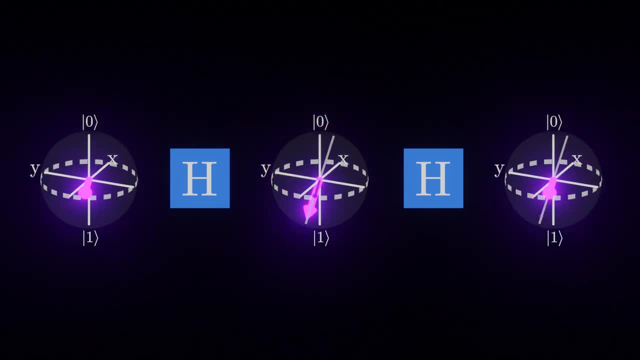 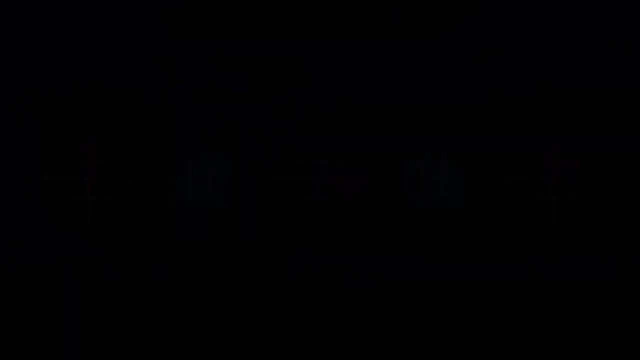 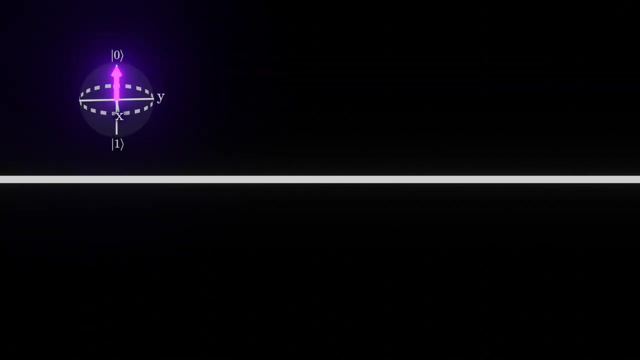 for why applying it twice seems to produce no change. In this video we looked at the behavior of individual qubits and how their states can be described by the Bloch sphere. We also explored how a variety of quantum logic gates can be described as rotations on the Bloch sphere. 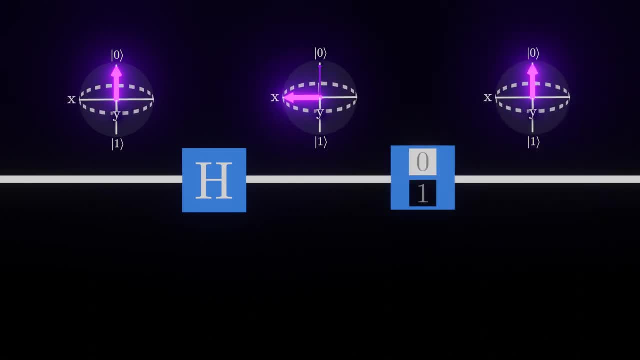 and how the measurement gate collapses qubits down to one of two states. The fact that individual qubits work in this way is pretty interesting, but by itself it doesn't let us do anything that we can't do with regular computers. In the next video. 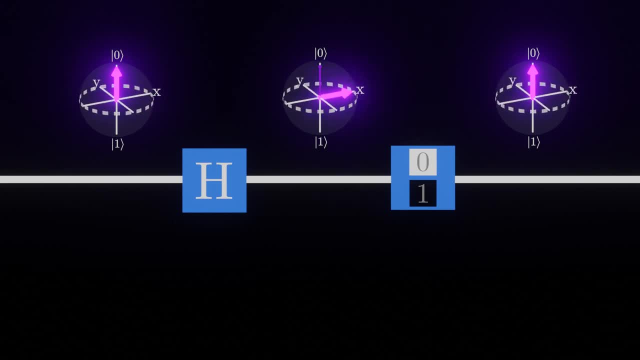 we'll look at the workings of entanglement and see how using multiple qubits at once lets us quickly perform operations on exponentially more data.